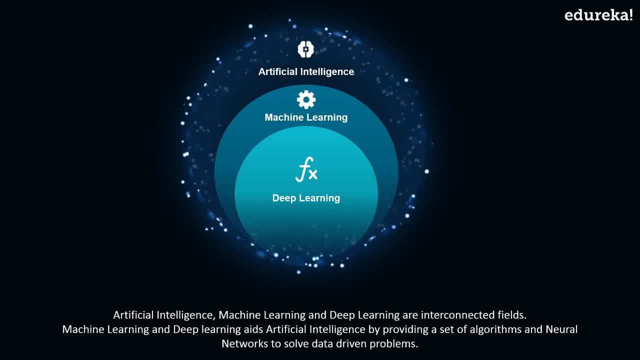 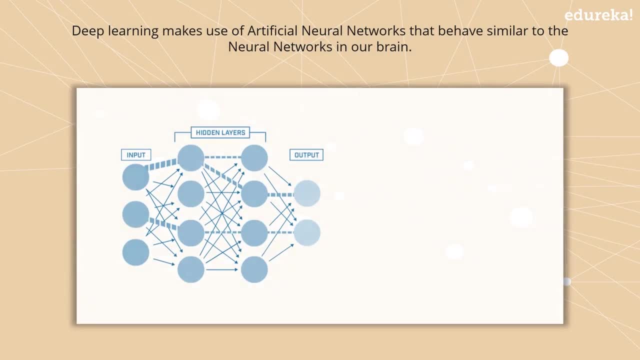 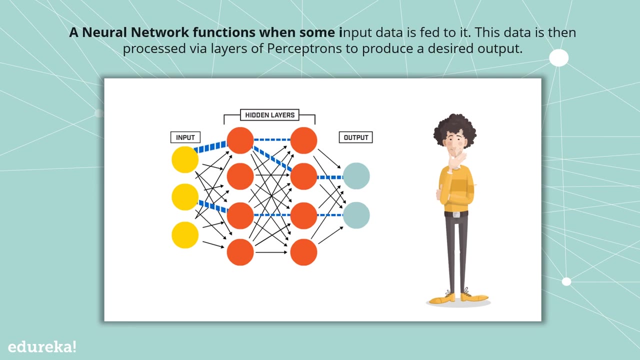 deep learning aids artificial intelligence by providing a set of algorithms and neural networks to solve data-driven problems. Deep learning makes use of artificial neural networks that behave similar to the neural networks in our brain. A neural network functions when some input data is fed to it. Now, this data is then processed via layers of perceptrons to produce 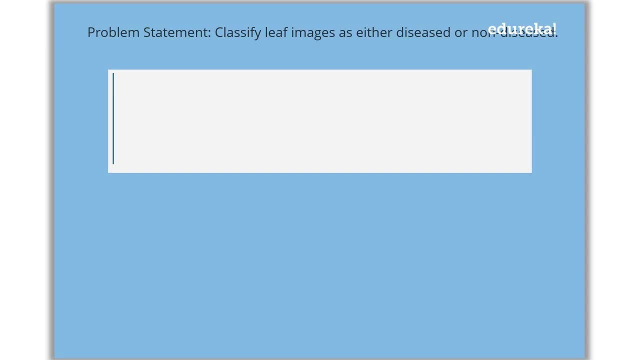 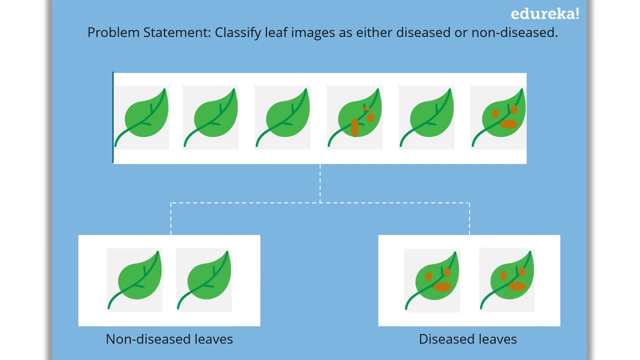 a desired output. So let's understand neural networks with a small example. Now consider a scenario where you have been given a set of labeled images and you have to classify them into two classes: One class containing images of non-diseased leaves and the other class containing 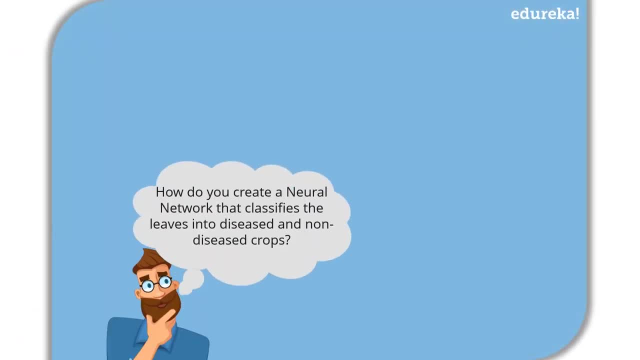 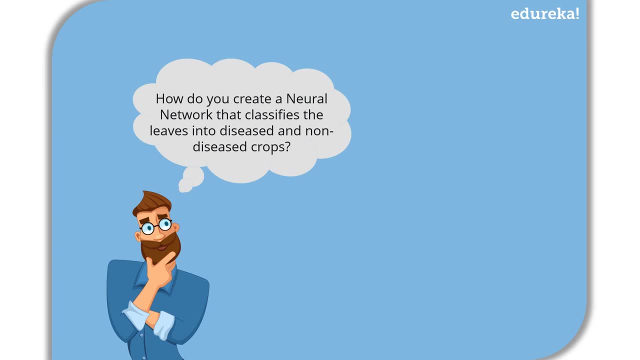 images of diseased leaves. So how would you create a neural network that classifies the leaves into diseased and non-diseased crops? Now, the process always begins with processing and transforming the input in such a way that it can be easily processed. In our case, each leaf image will be. 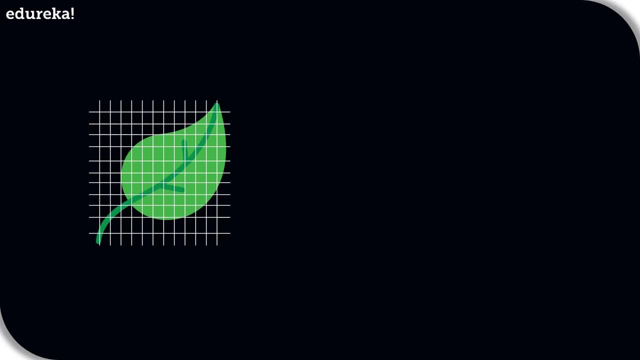 broken down into pixels, depending on the dimension of the image. So let's say that we have a leaf image and we want to classify it into the dimension of the image. For example, if the image is composed of 30 by 30 pixels, then the total 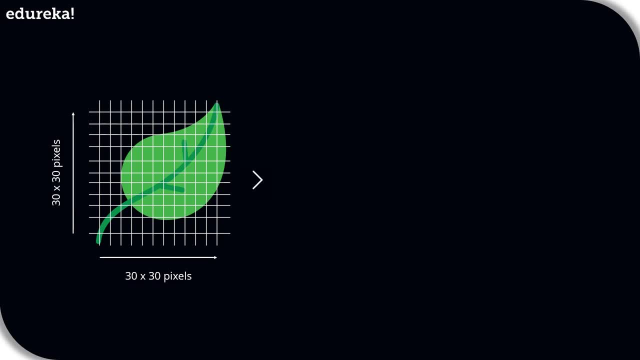 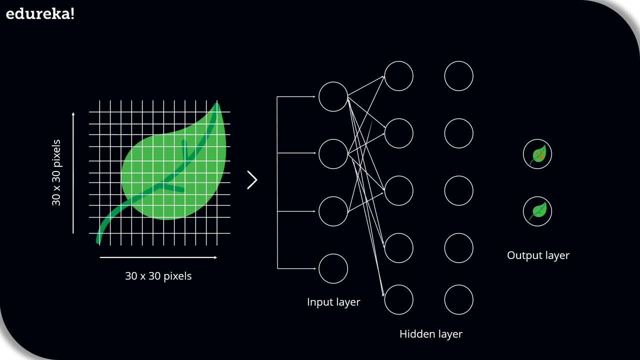 number of pixels will be 900.. Now these pixels are represented as matrices, which are then fed into the input layer of the neural network. Just like how our brains have neurons that help in building and connecting thoughts, an artificial neural network has perceptrons that accept inputs. 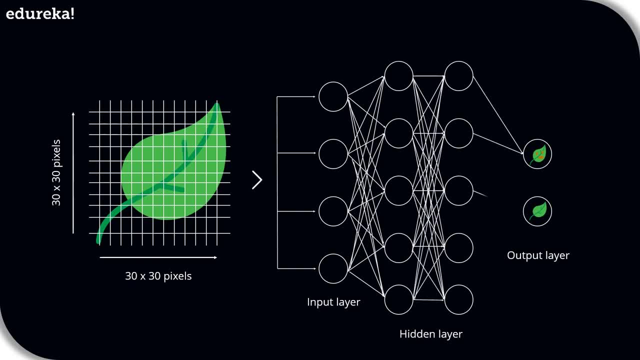 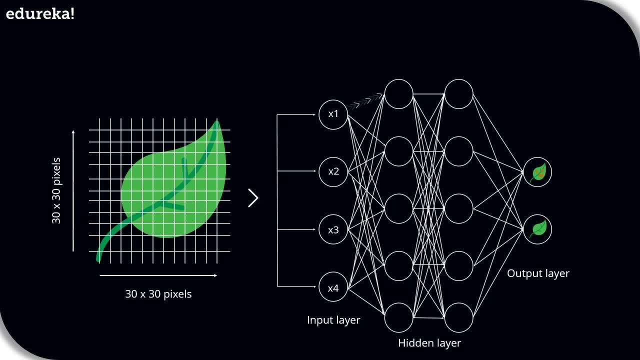 and process them by passing them on from the input layer to the hidden and finally, the output layer. Now, as the input is passed from the input layer to the hidden layer, an initial random weight is assigned to each input. The inputs are then multiplied with their 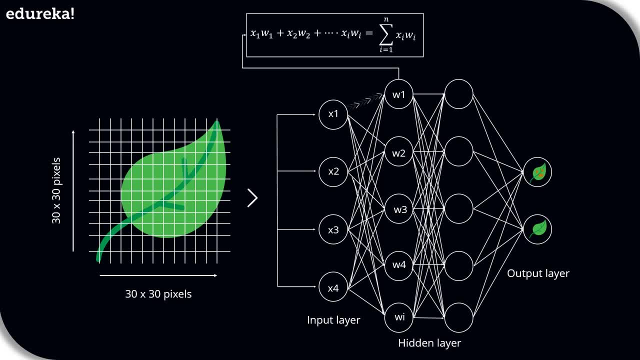 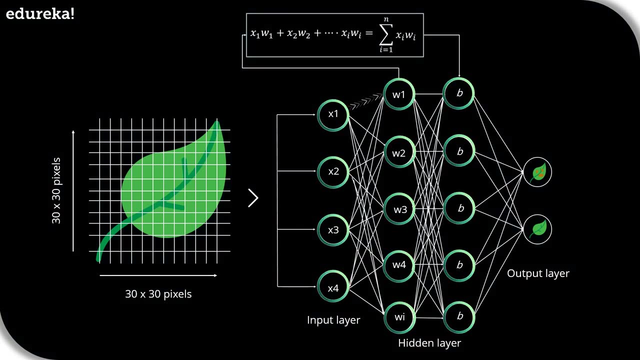 corresponding weights, and their sum is further processed through the network. Now, here, what you do is you assign a numerical value, called bias, to each perceptron. Furthermore, each perceptron is passed through activation, or something known as the transformation function. that determines whether a particular perceptron gets activated or not. 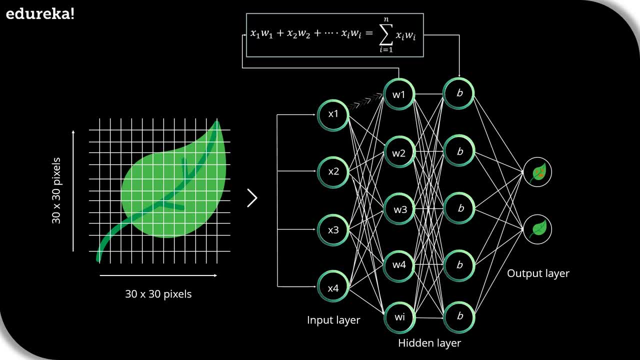 An activated perceptron is used to transmit data to the next layer. In this manner, the data is propagated forward through the neural network until the perceptrons reach the output layer. At the output layer, a probability is derived which decides whether the data belongs to class. 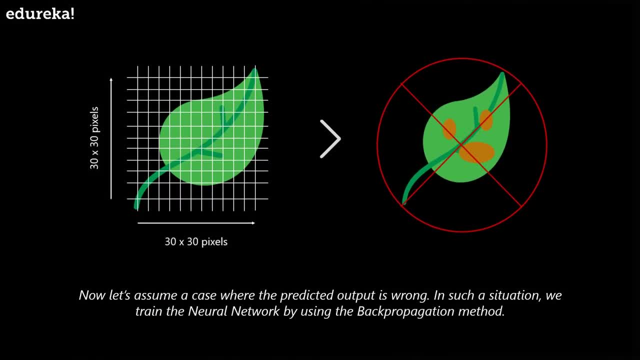 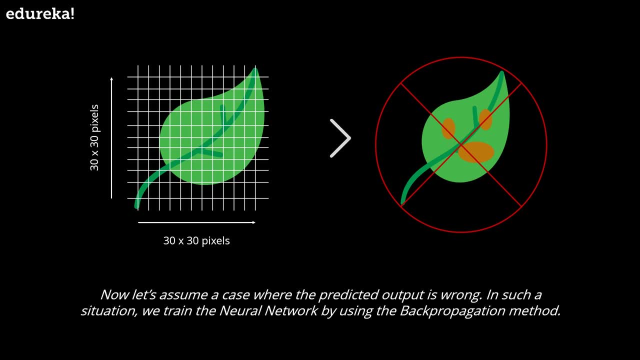 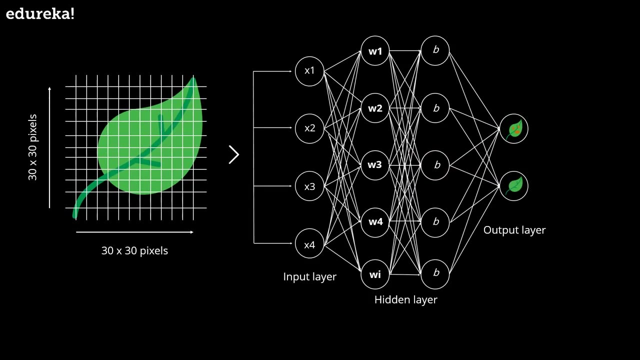 A or class B. Now let's assume a case where the predicted output is wrong. In such a situation, we train the neural network by using the back propagation method. Initially, while designing the neural network, we initialize weights to each input with some random values. Now these weights denote: 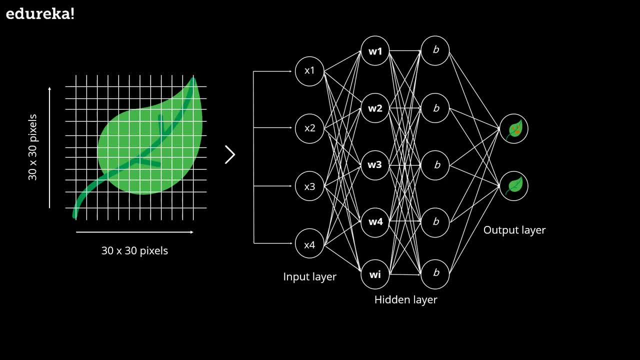 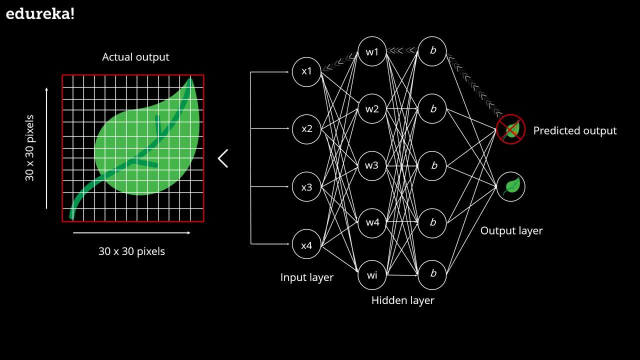 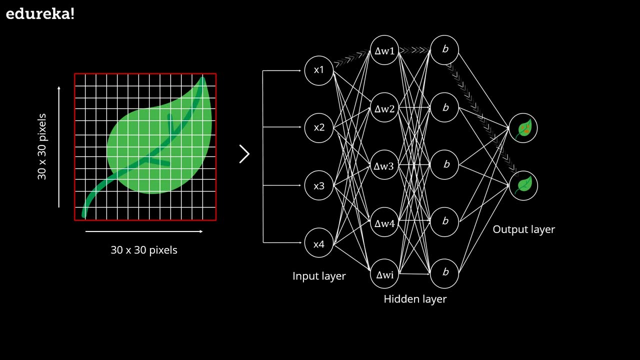 the importance of each input variable. Therefore, if we propagate backward in a neural network and compare the actual output to the predicted output, we can readjust the weights of each input in such a way that the error is minimized. This results in a more accurate output, and this is exactly what back propagation means. 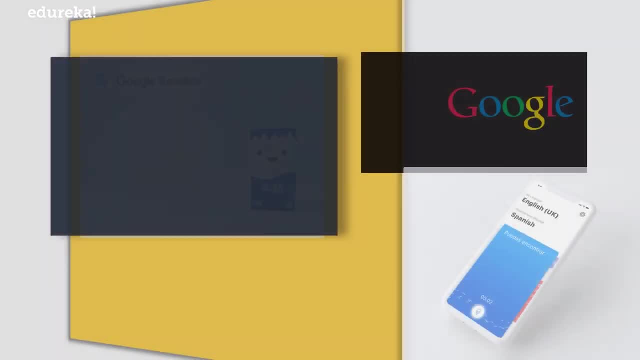 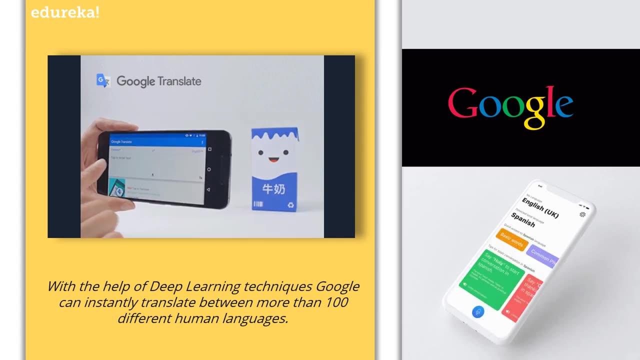 Now let's discuss a few real-world applications of neural networks. With the help of deep learning techniques, Google can instantly translate between more than hundred different human languages. Visual translation is an interesting application of deep learning. It can be used to identify images that have letters. Now, once you identify them, they can be turned into text translate. 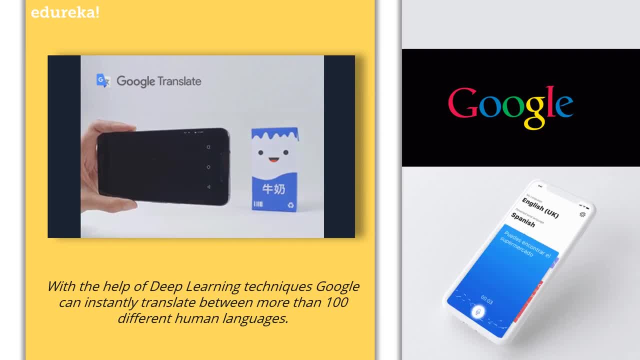 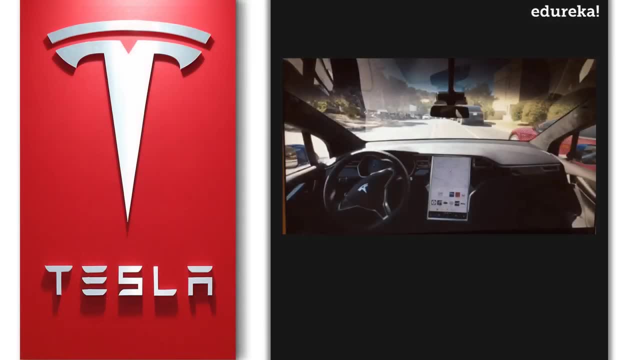 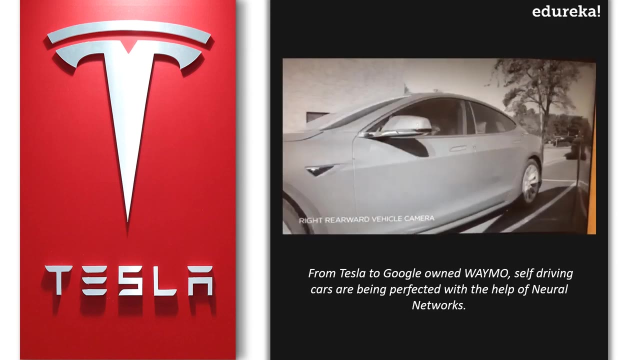 and then the images are recreated with a translated text. In fact, Google has an app for this purpose. It's called the Google Translate app. Let's not forget to mention automated self-driven cars. Deep learning has played a huge role in the field of self-driving cars, From Tesla to Google-owned Waymo. 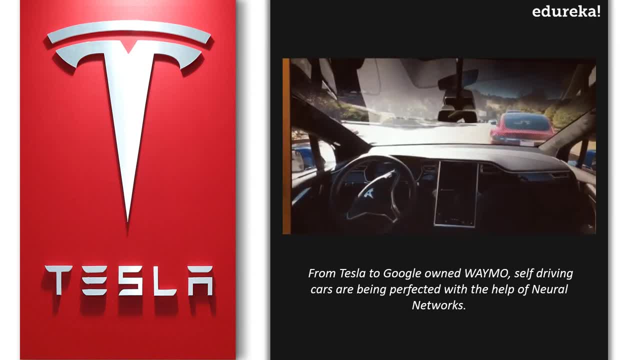 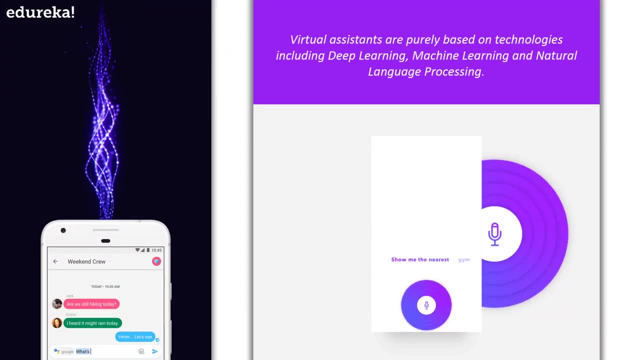 self-driving cars are being perfected with the help of neural networks. Then, of course, we have the virtual assistants, like Siri, Alexa Cortana, that can live and work in a virtual environment. You can literally read your mind. These assistants are purely based on technologies, including 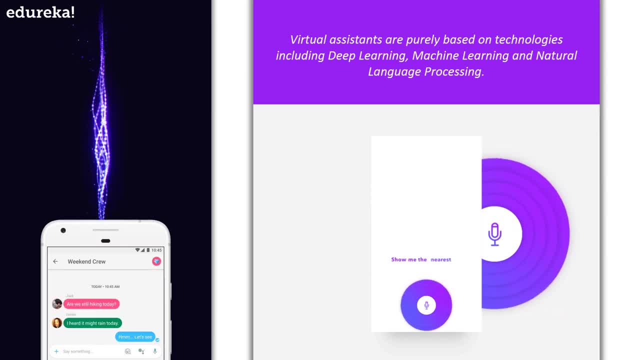 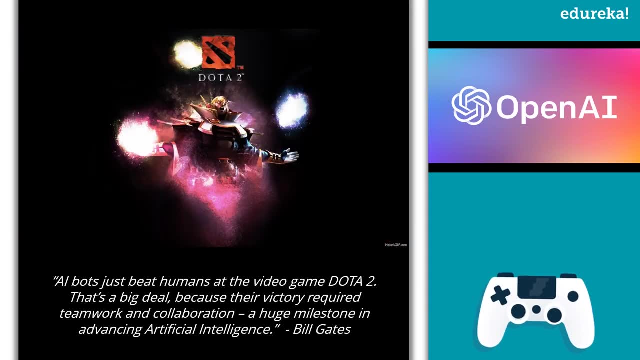 deep learning, machine learning and natural language processing. Apart from this, deep learning has also made its way into the gaming industry. So all you Dota fans out there might have already heard of the famous Open AI 5, which is the first AI to beat the world champions.